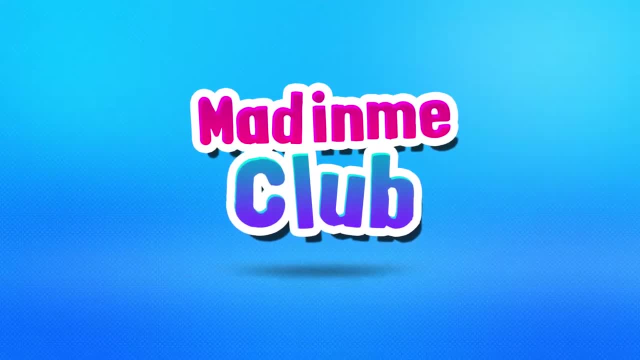 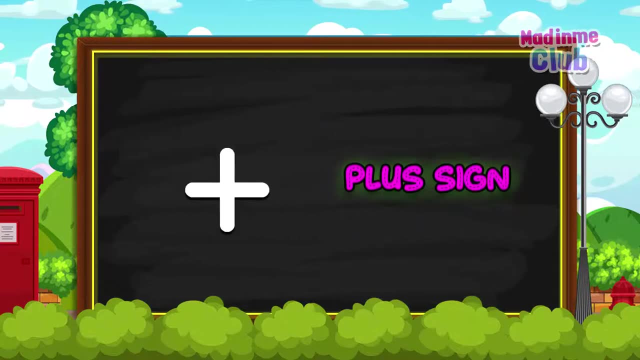 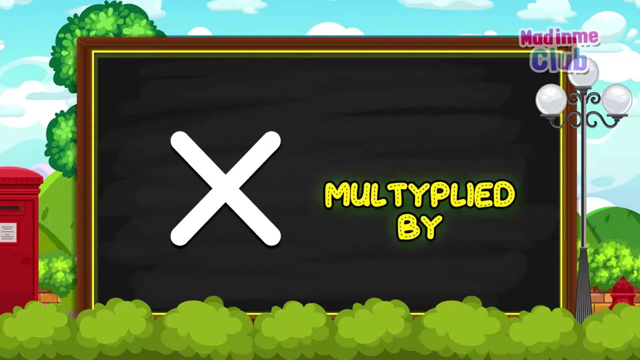 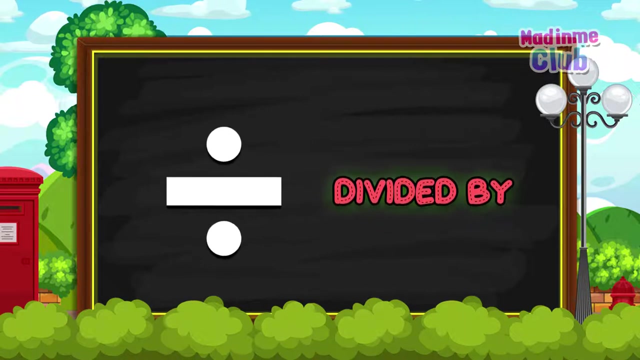 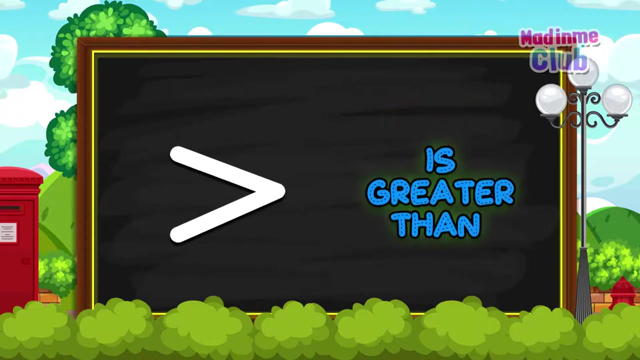 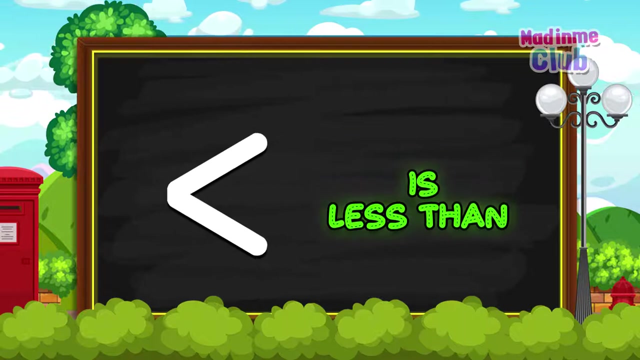 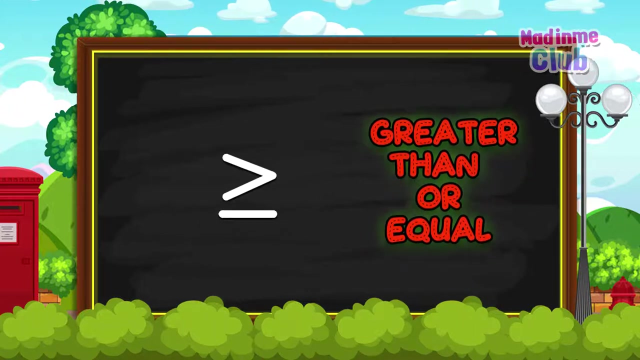 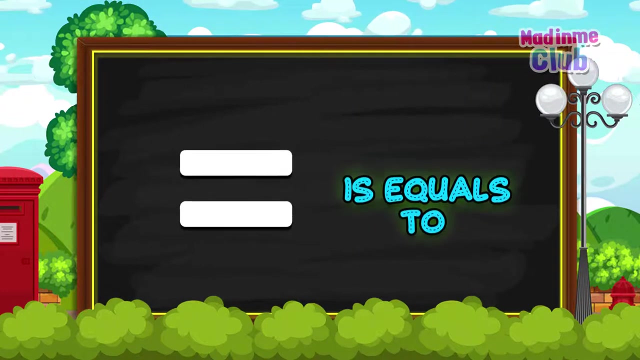 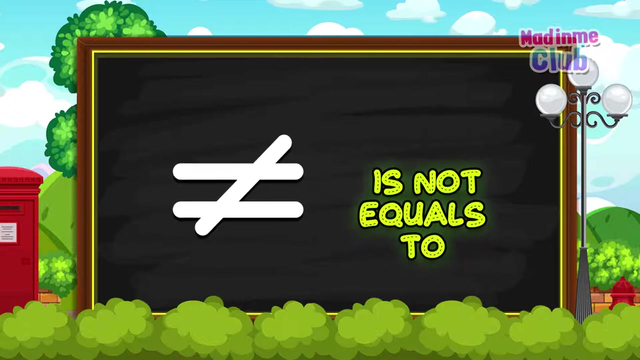 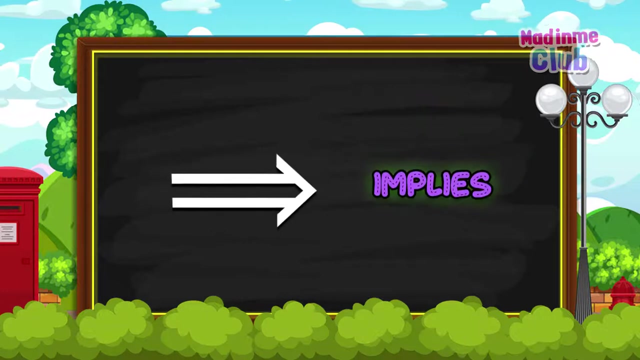 Plus sign. Minus sign. Multiplied by Divided by Plus or minus, Is greater than, Is less than. Greater than or equal. Less than or equal. Is equals to, Is not equals to. Is equivalent to Implied. 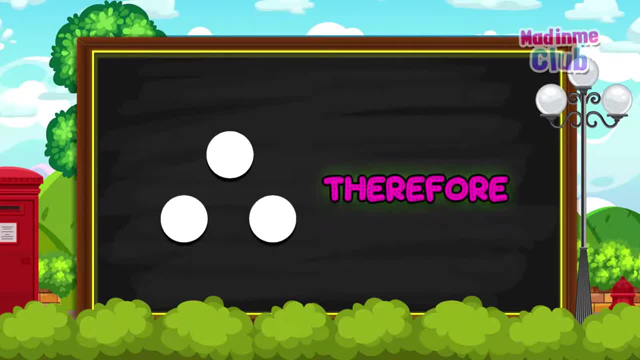 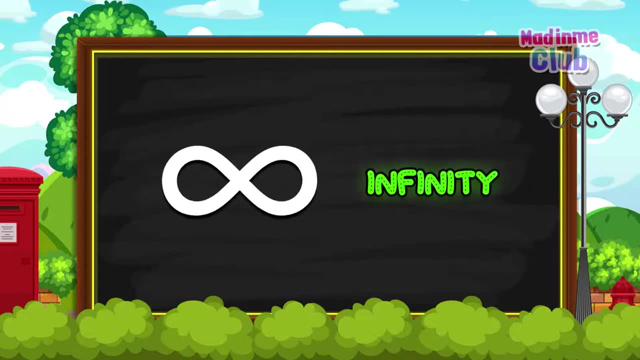 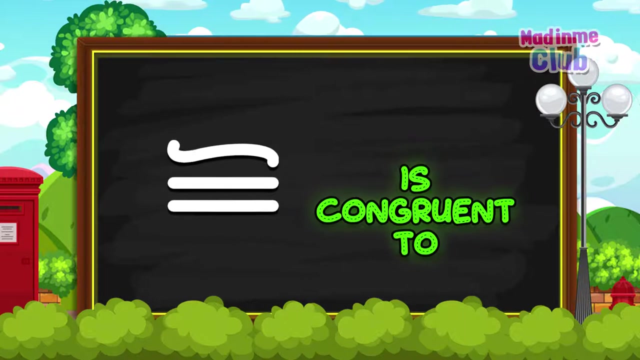 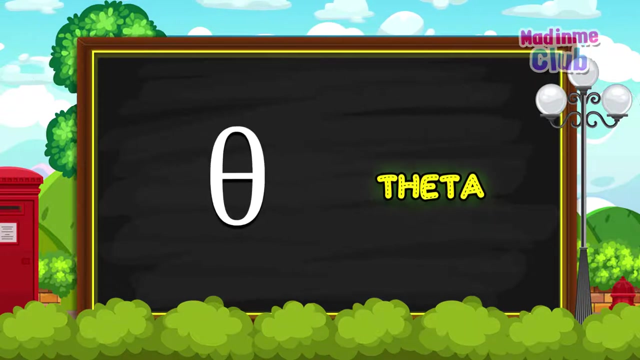 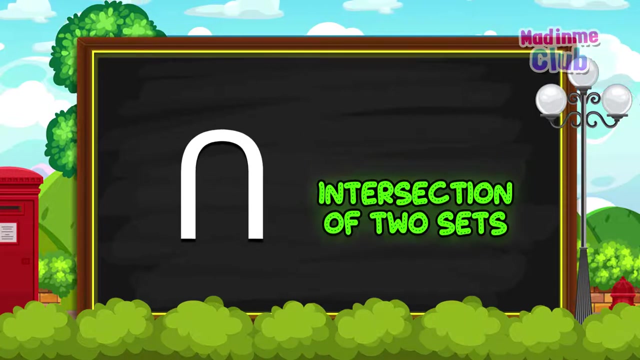 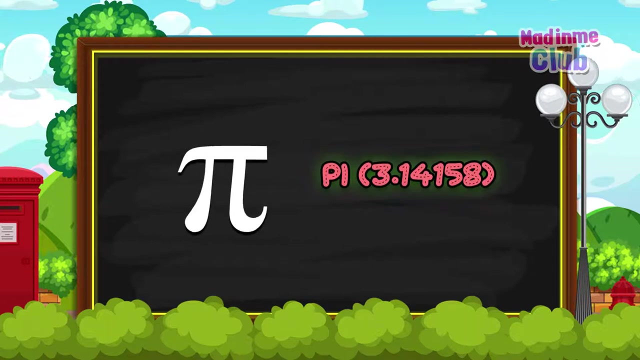 Therefore, Since Infinite Percent Is similar to Approximately equal, Is congruent to Theta Square. root of Perpendicular Parallel Empathy set. Union of two sets, Intersection of two sets, Pi, Sum of Angle. 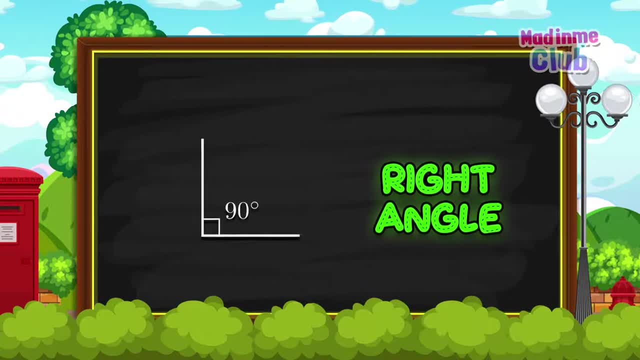 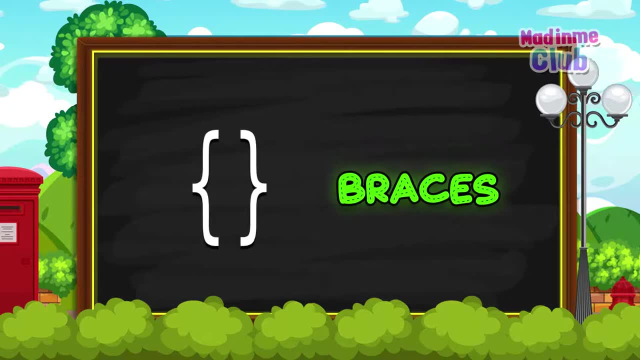 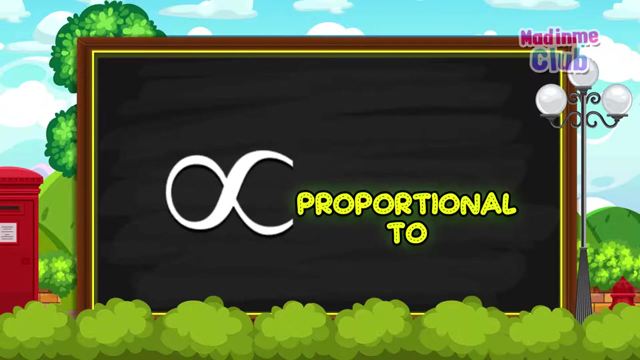 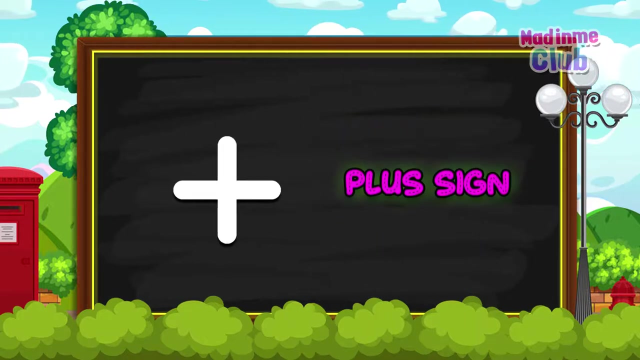 Right angle Triangle of delta Braces, Parentheses, Brackets. Integral. Proportional to Degree. Factorial For all: There exists. There dones not exists. Plus sign, Minus sign Multiplied by: 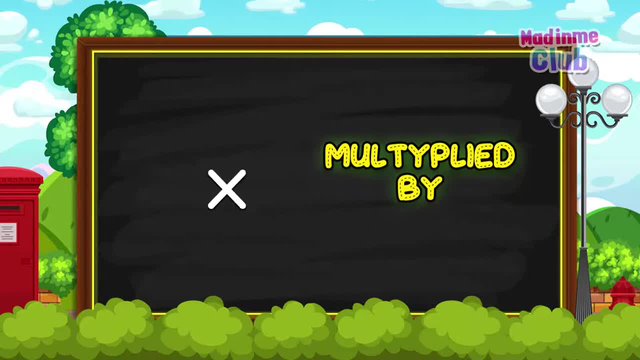 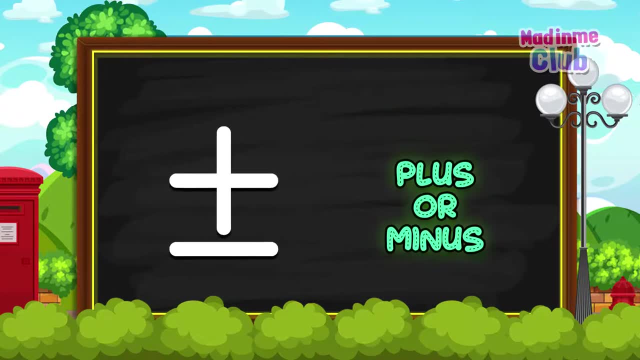 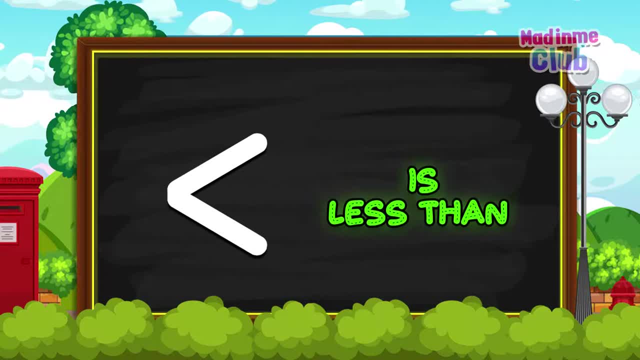 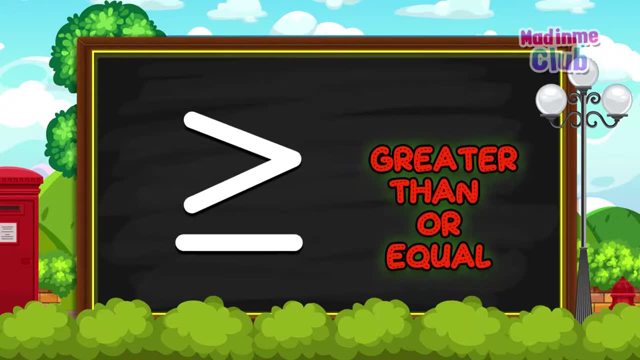 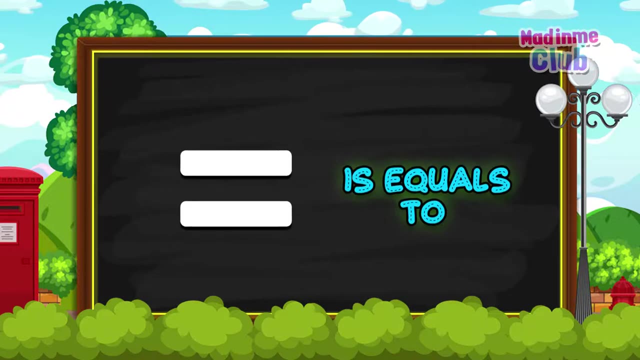 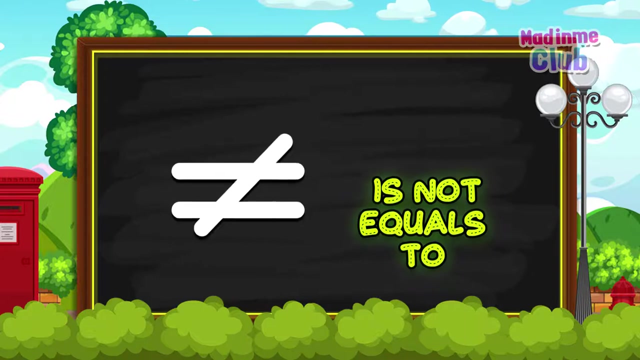 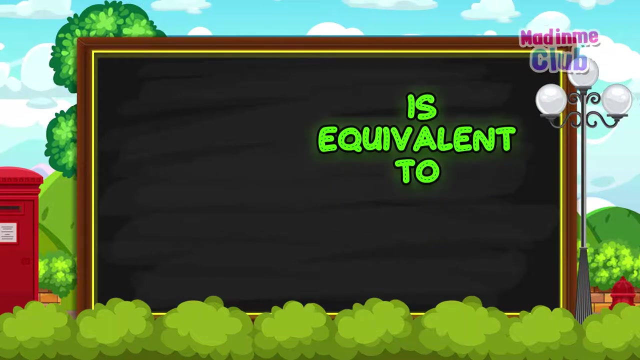 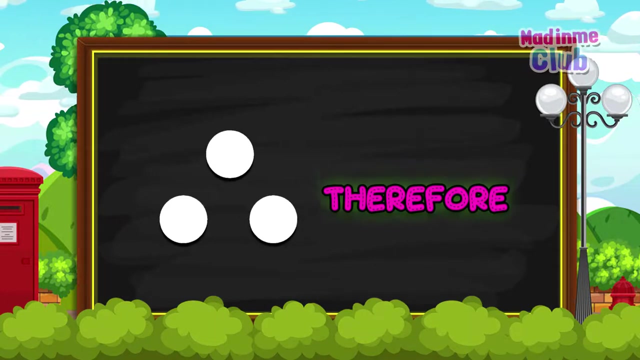 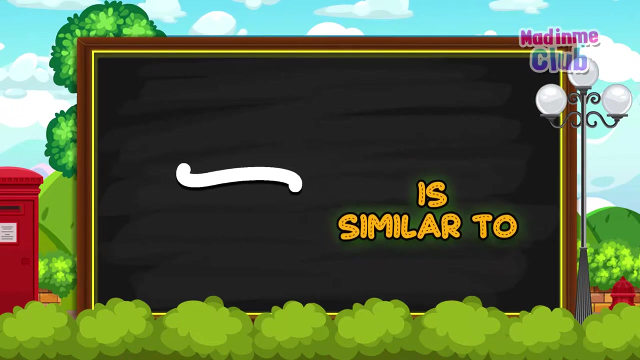 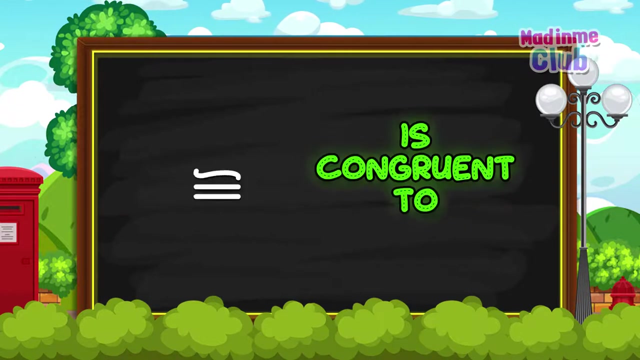 Simple Perfect to Public is equal to is equal to bard And humble A son, Then等 to is equivalent to implied. therefore, since infinite percent is similar to approximately equal is congruent to theta square root of perpendicular parallel empty set. union of two sets.